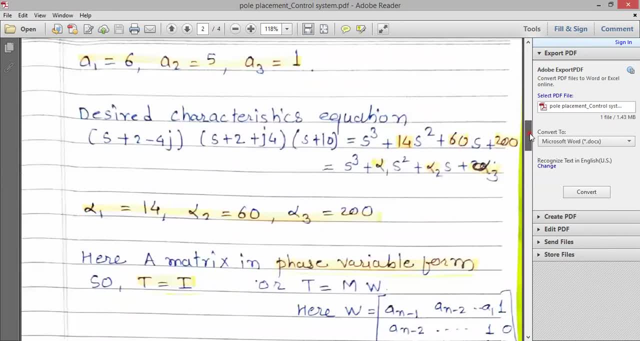 the value. Next step is get the desired closed loop poles. So that is a rank equal to N, So that is a characteristic equation. So to finding the desired characteristic equation, So this is using desired poles, or the closed loop poles. get the values, So this is a desired characteristic. 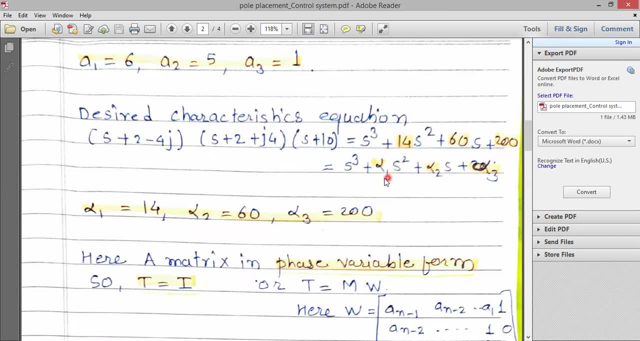 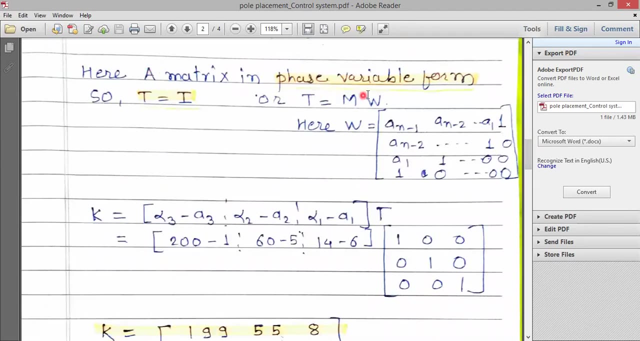 equation. Now compare with the standard equation and get the coefficient alpha 1, alpha 2 and alpha 3.. So like this comparison. Next step is a phase variable form checker. So this is a phase variable. if the given a matrix is in the phase variable form, controllable canonical form, that time t. 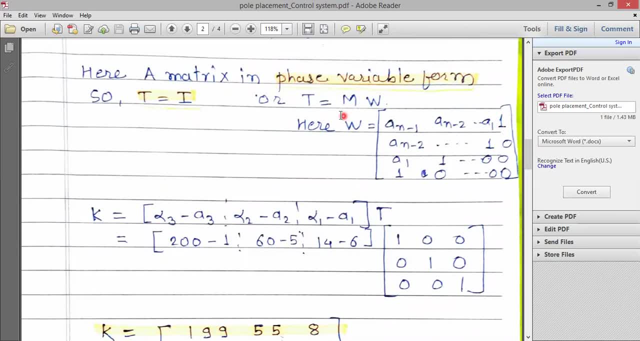 matrix equal to i. so that is identity. otherwise we have to calculate the t matrix. so that is m into w. m is a kalman matrix and w is. this is a standard w matrix. we have to replace it by the a1, a2 coefficients, but here, given a matrix is in the phase variable form, so t is equal to i. 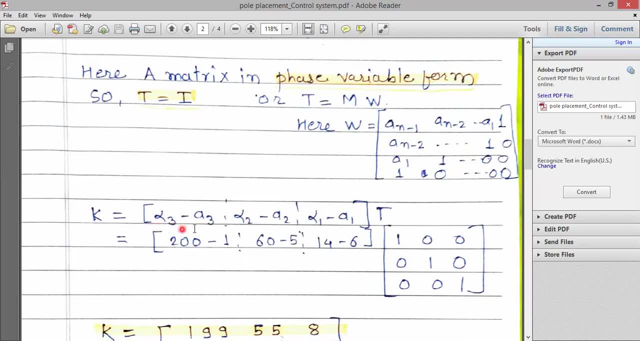 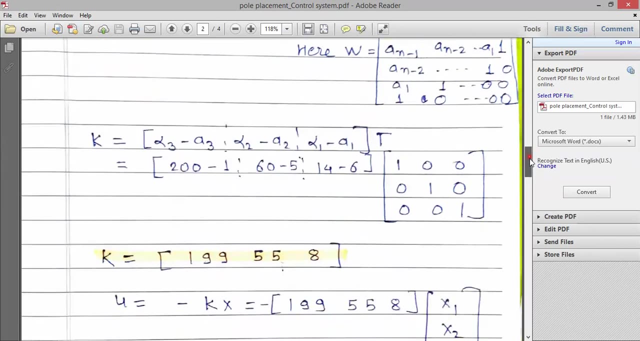 and these are the standard equation to get the k matrix. so alpha 3 minus a3, a2 minus a1, alpha 1 minus a1. so in this way we have to just do the subtraction and multiply by the t matrix. so here t is equal to i. 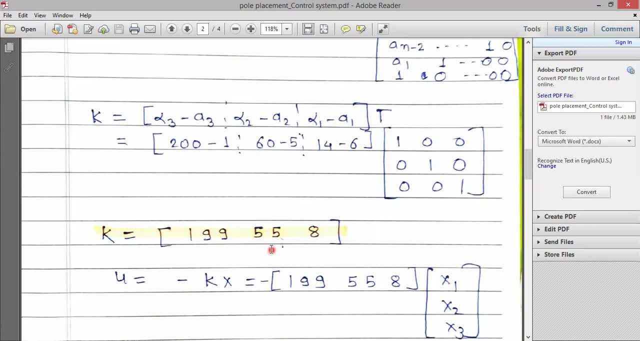 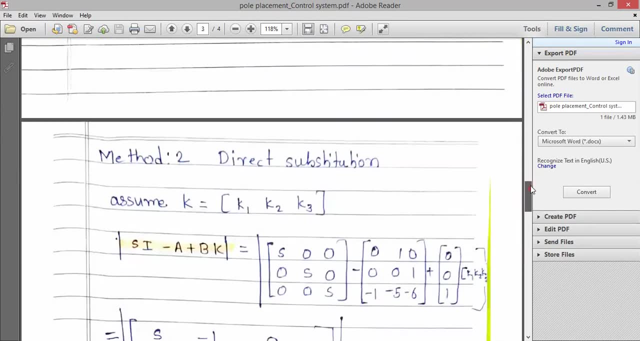 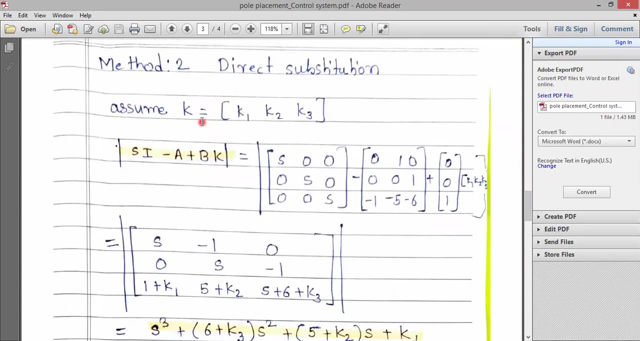 so this is the calculated k matrix will have the three coefficient. so this is first method to get the transformation matrix, to finding the k matrix. second method is a direct substitution method. so we have to assume the k equal to k1, k2, k3 and get the determinant of si minus a plus bk. 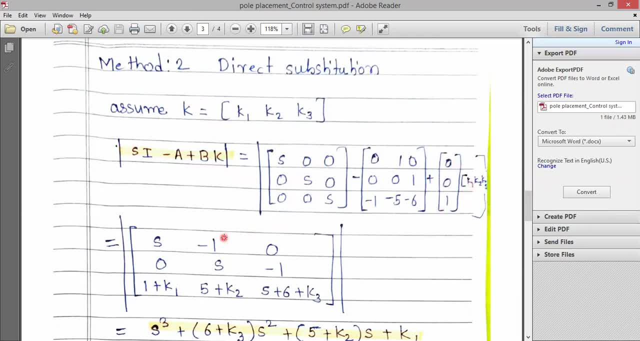 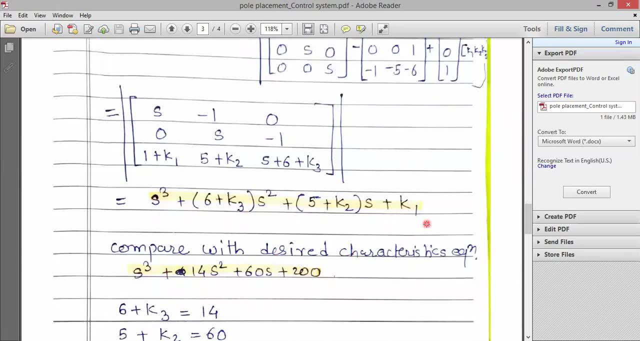 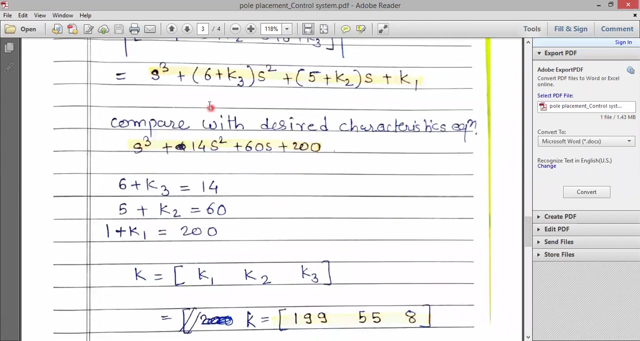 just find out the this new matrix, so that is a si minus a plus bk, and get the determinant equation, or we can say the characteristic equation. compare this with the desired characteristic equation that we calculated already using the given desired values, eigenvalues. then when we compare the coefficients, so this: 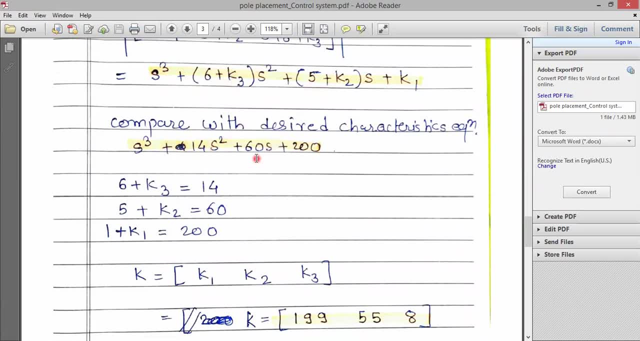 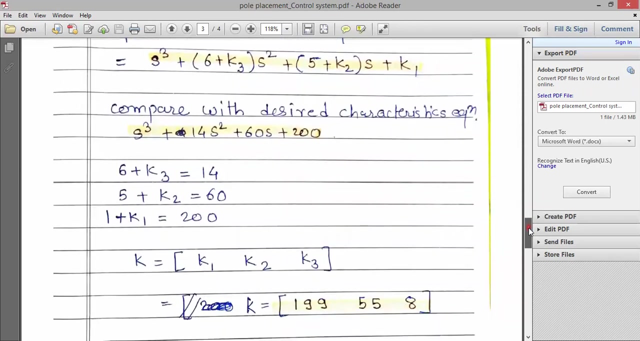 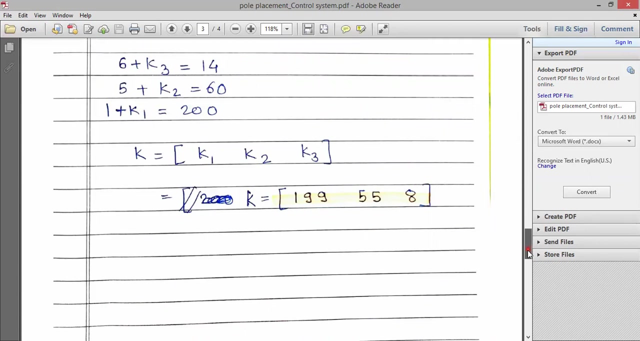 3 plus c with 14, this with the 60 and this with the, we can say the 200.. so when we compare these, so we get the values in terms of characteristic equation. so then, same value, we calculated 199, 55 and 8. next method, third method, is a occurrent formula. 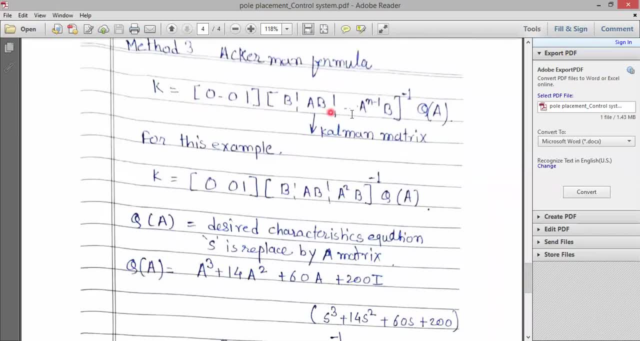 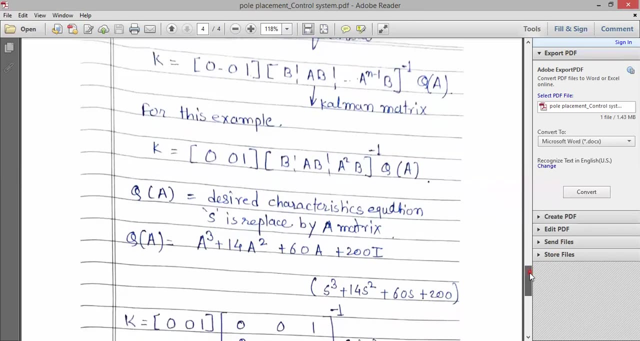 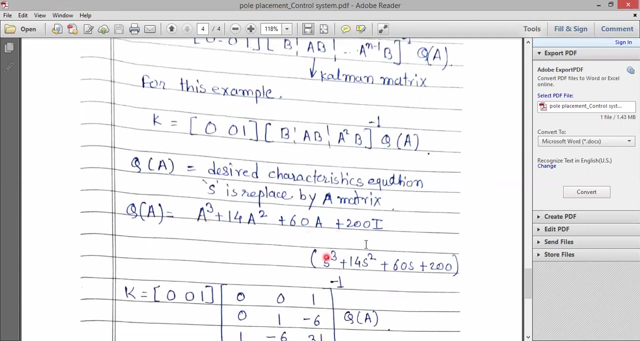 so occurrent formula is standard formula. this is the kerman formula. kalman matrix inverse into qa. so that is a desired characteristic equation with respect to that given system matrix. then whenever the s is there, we have to replace by the a and this is the characteristic equation. now, your family, this is the characteristic. 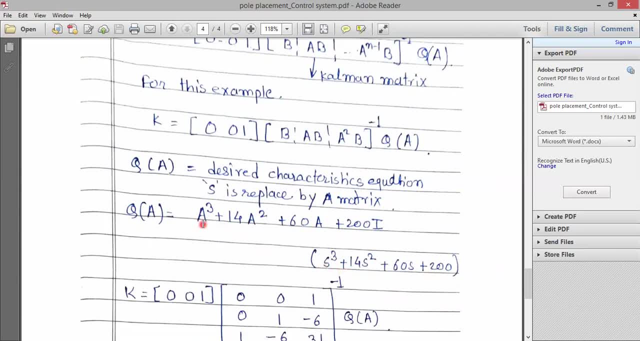 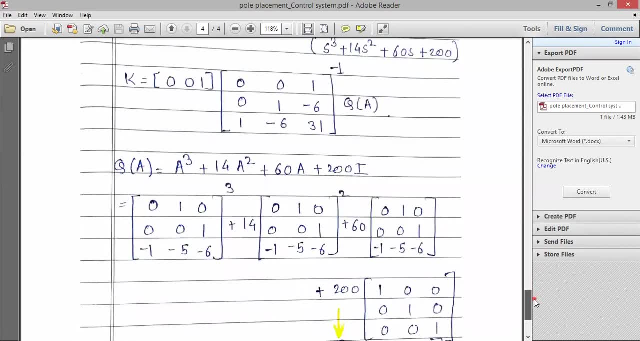 equation whenever s is there, replaced by the a value, so you will get the matrix equation. now put the the this equation as it is, then this is the kalman matrix. we take the inverse and then multiply by the characteristic matrix equation. calculate this matrix equation of finding the a cube, a square a, and multiply by this. 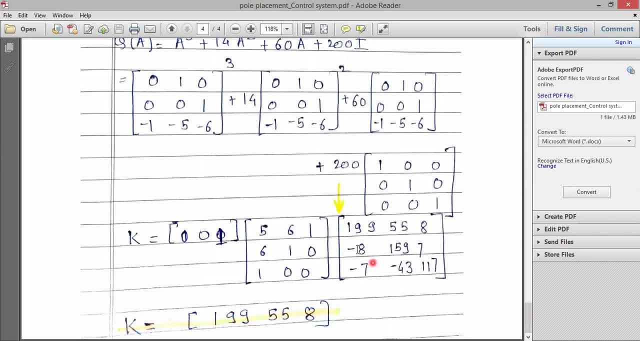 respectively coefficient. so this is calculated equation. then this is the inverse of that kalman matrix and when we do the all multiplication you will get the desired k matrix. so k is a feedback gain matrix. so by choosing any method you can find out the k matrix for the pole placement method. 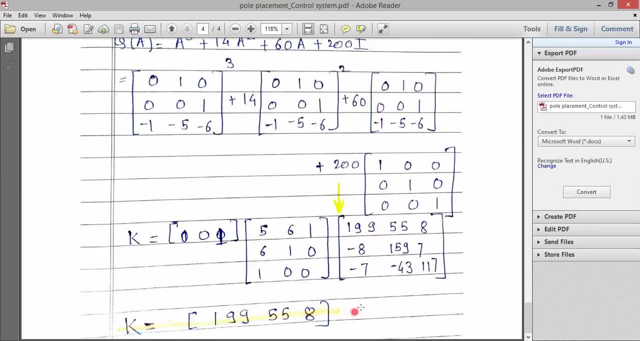 thank you, hope you understand all three methods. 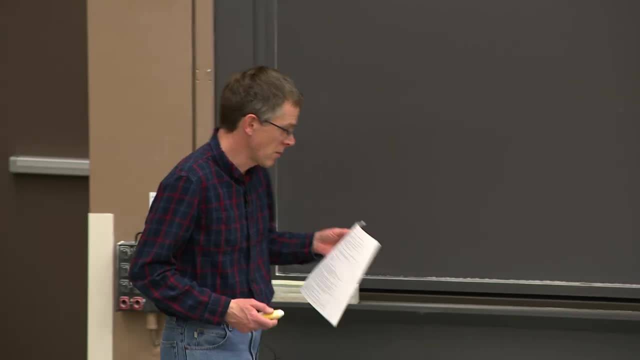 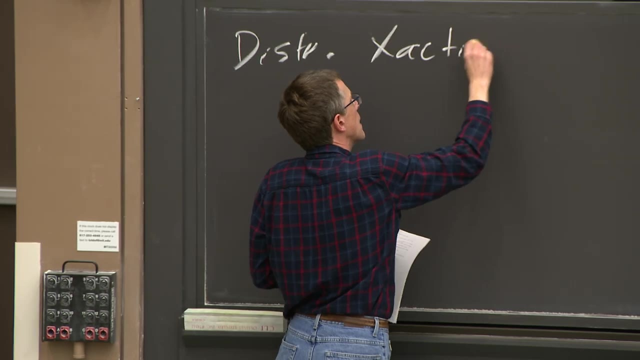 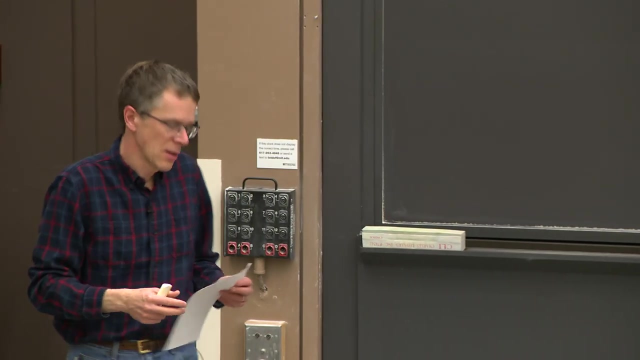 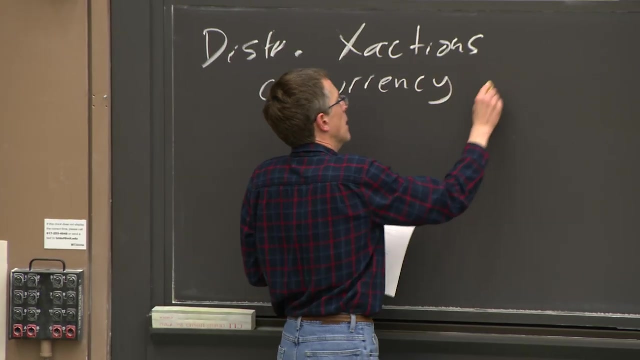 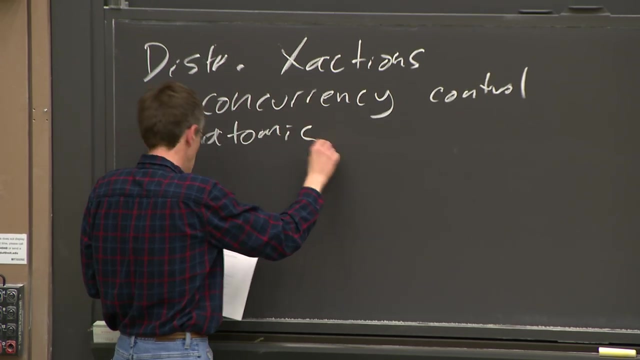 All right. today's topic is distributed transactions and these come in really two implementation pieces, and that's how I'll cover them. The first big piece is concurrency control, The second is atomic commit, And the reason why distributed transactions come up is that it's very frequent for people with large amounts of data to end up splitting or sharding the data over many different servers. So maybe if you're running a bank, for example, the bank balances for half of your customers are one server and the other half of your customers are one server.